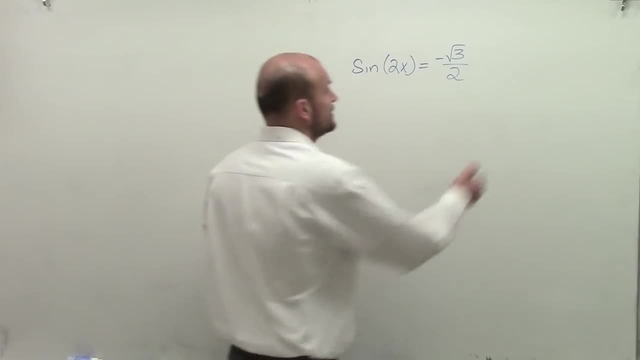 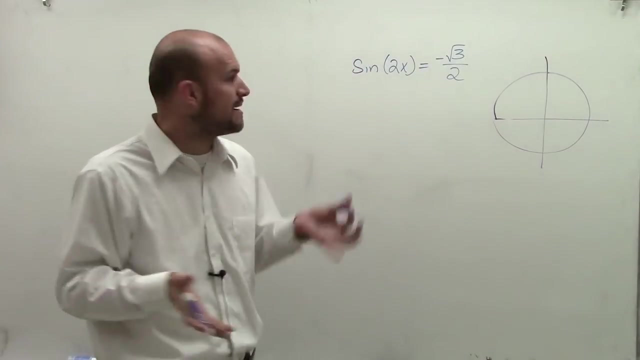 is find at least the solutions that are going to be on the interval of 0 and 2 pi. So again, I'll create my unit circle here. All right, so now what I want to do is determine when are my values of my sine of an angle? 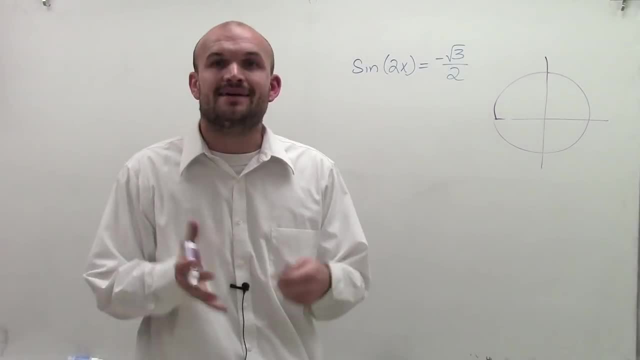 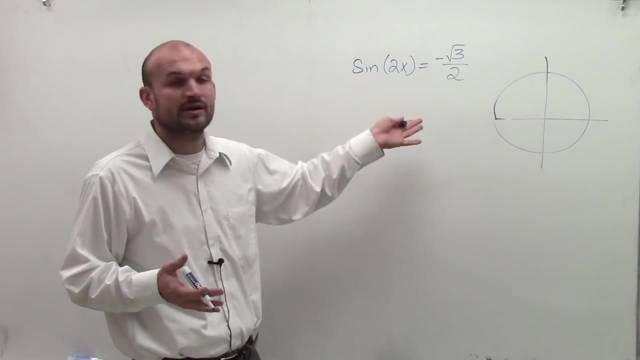 equal to negative square root of 3 over 2.. Now remember that when looking at the unit circle, the sine of an angle is equal to the y-coordinate of that coordinate point of your angle on the unit circle. So I need to look over here and now. 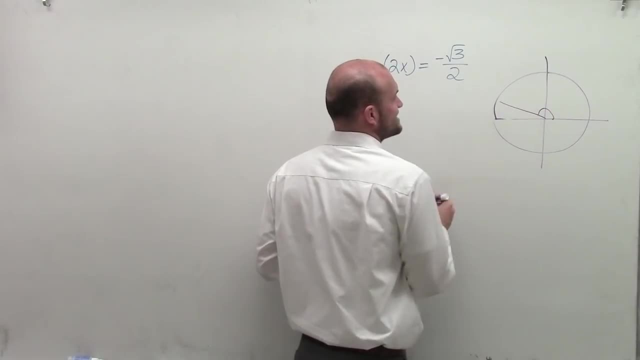 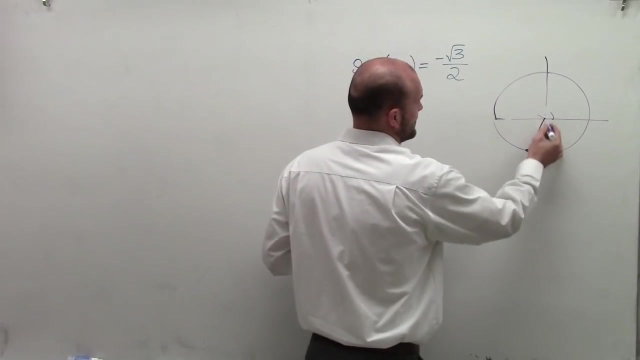 determine that there's two angles, that when my sine is equal to a negative square root of 3 over 2. Well, we can look at this and say it's going to be here and roughly here. All right, now, that's not the best. 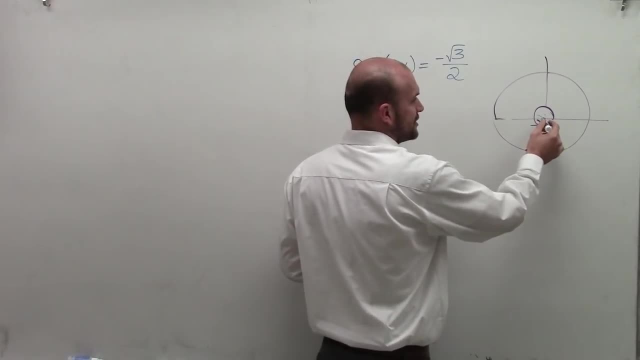 that you can look at this, But what I did is these are on my thirds. If I said 1 third, 2 thirds, 3 thirds, then this would be 4 thirds, 5 thirds and then 6 thirds. 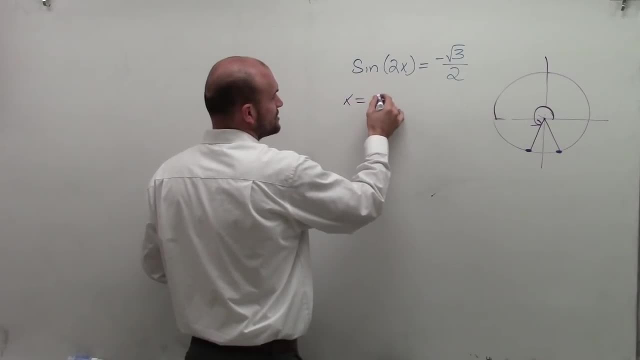 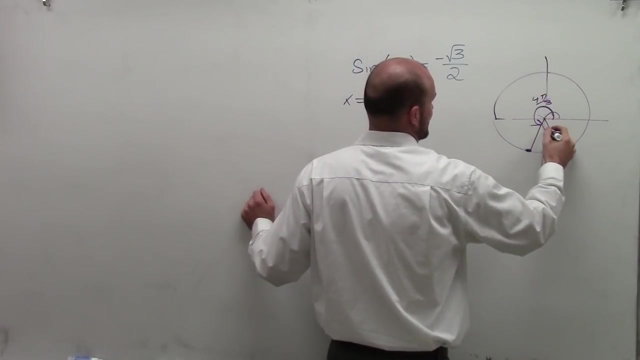 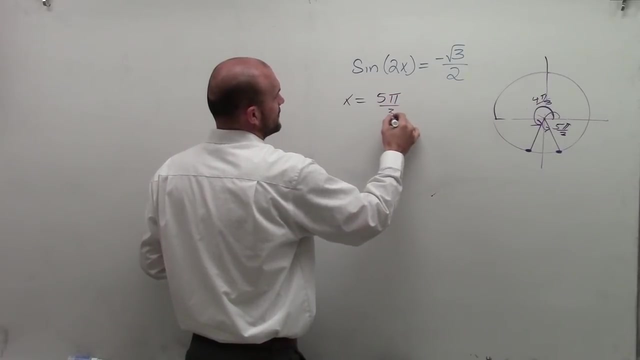 So we're going to have- we could say, x equals the angle. This first angle we're going to call is 4 pi over 3.. And then the next angle is going to be 5 pi over 3.. So we could say x equals 5 pi over 3 and x equals 4 pi over 3.. 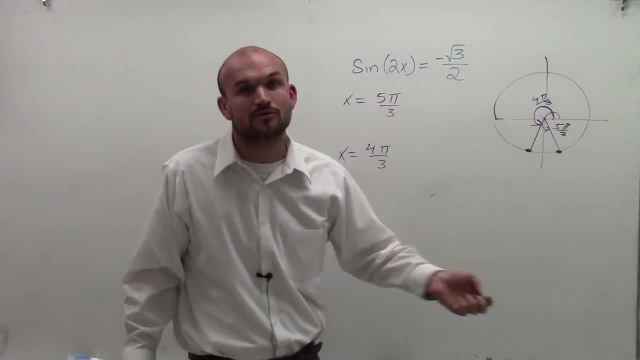 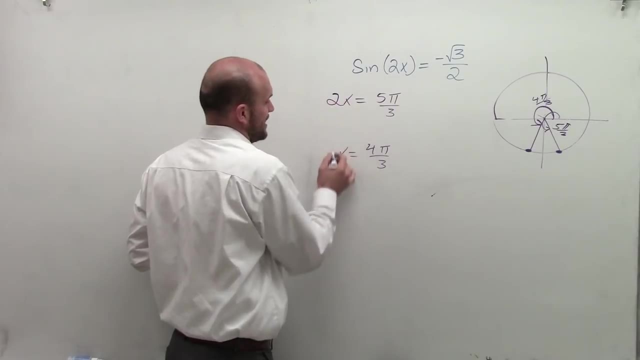 So those are the two angles. when I take the sine of an angle and it's equal to a negative square root of 3 divided by 2.. However, we're not trying to find the angle of just x, It's actually 2x. 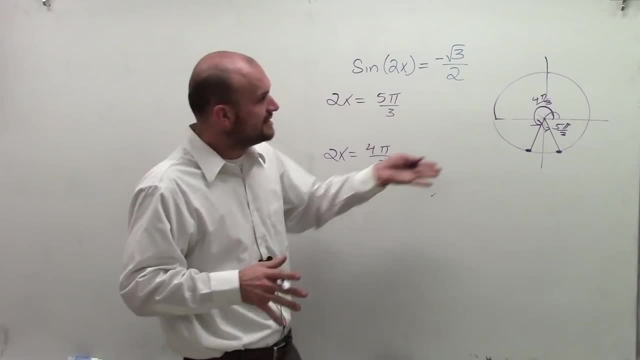 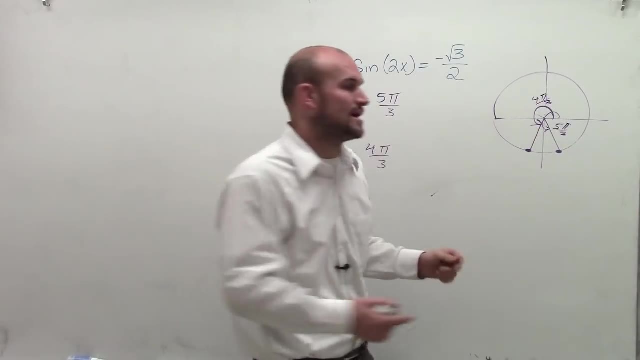 All right, so then, the next thing that we need to look at this is: these are my two angles that are on the interval of 0 and 2 pi. But notice, we want to find all the solutions, So we're going to keep on adding and subtracting our coterminal. 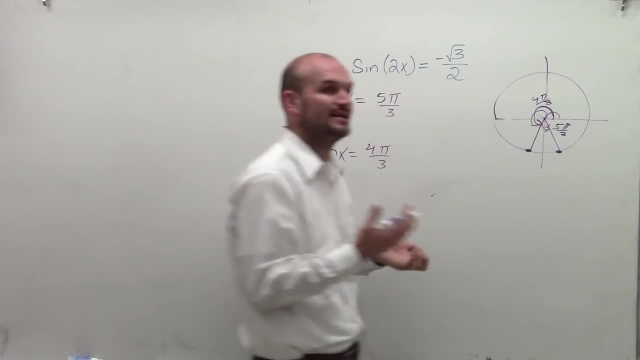 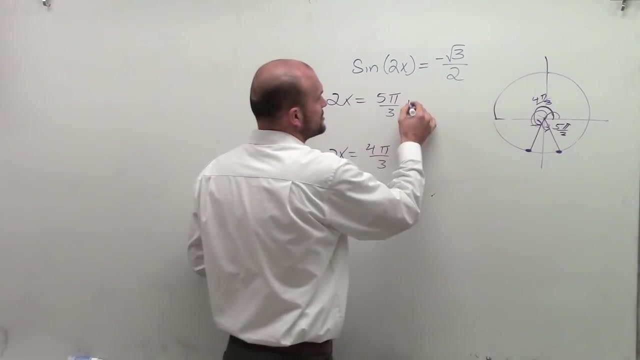 angles, because we can keep on going around and around and keep on getting the solutions of sine being negative- square root of 3 divided by 2, as long as we don't limit it between 0 and 2 pi. So to find my next angle, I can add 2 pi. 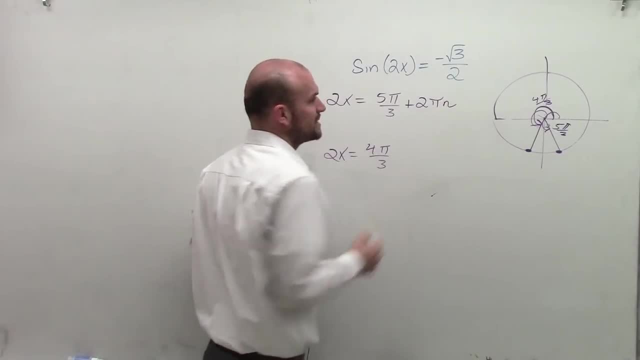 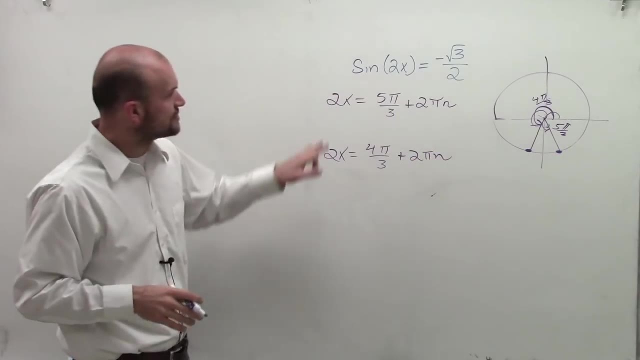 And I can keep on doing this infinite many times, And so therefore I'm going to leave it as a variable. n. Then I can also do the same thing with 2 pi and as well over here. So now to finally solve for x what I'll do. 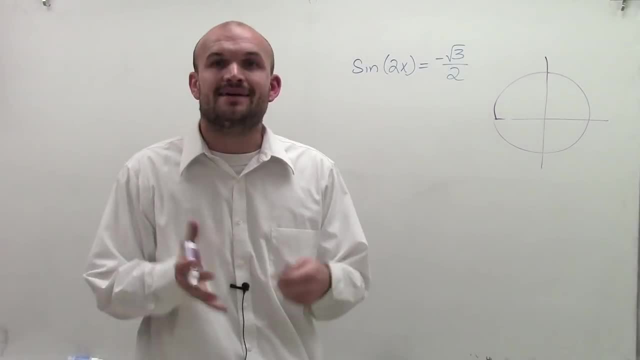 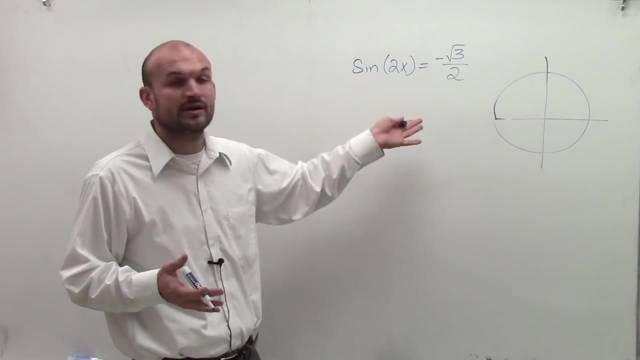 equal to negative square root of 3 over 2.. Now remember that when looking at the unit circle, the sine of an angle is equal to the y-coordinate of that coordinate point of your angle on the unit circle. So I need to look over here and now. 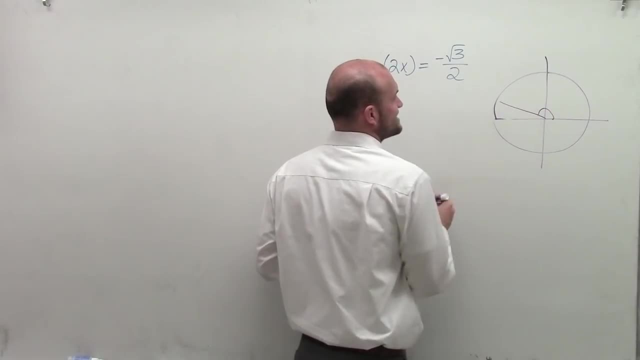 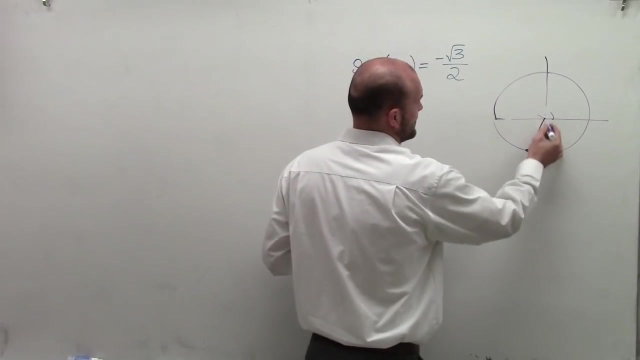 determine that there's two angles, that when my sine is equal to a negative square root of 3 over 2. Well, we can look at this and say it's going to be here and roughly here. All right, now, that's not the best. 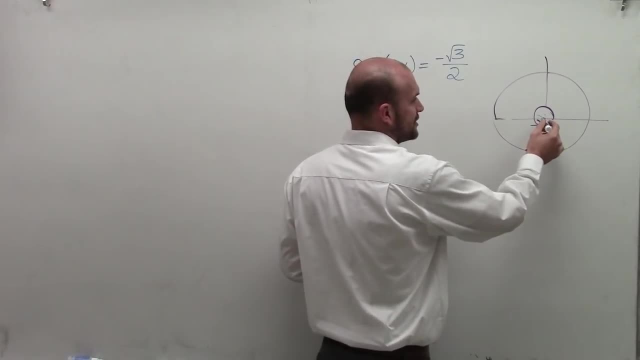 that you can look at this, But what I did is these are on my thirds. If I said 1 third, 2 thirds, 3 thirds, then this would be 4 thirds, 5 thirds and then 6 thirds. 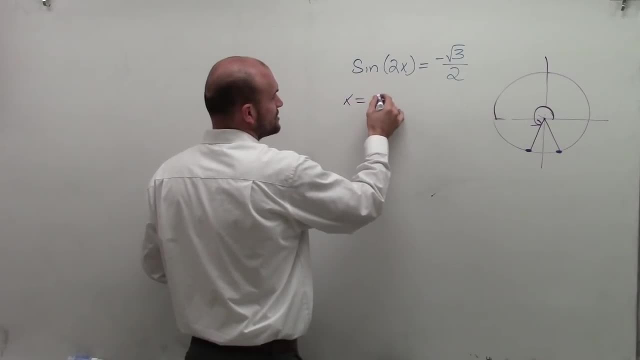 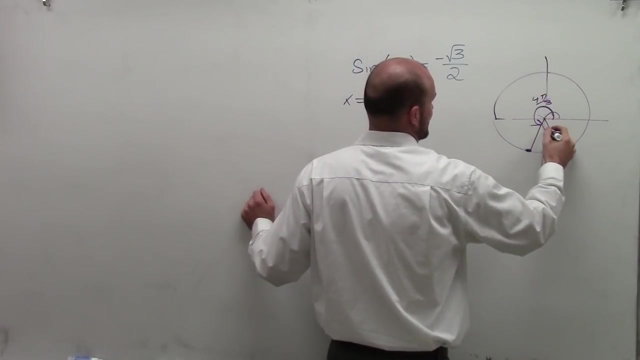 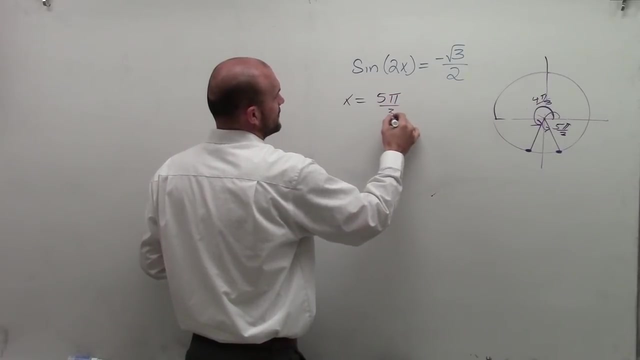 So we're going to have- we could say, x equals the angle. This first angle we're going to call is 4 pi over 3.. And then the next angle is going to be 5 pi over 3.. So we could say x equals 5 pi over 3 and x equals 4 pi over 3.. 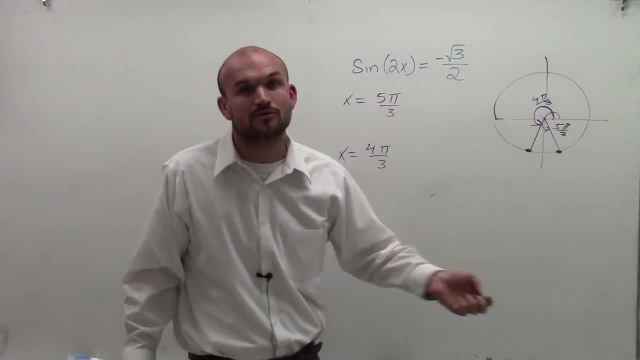 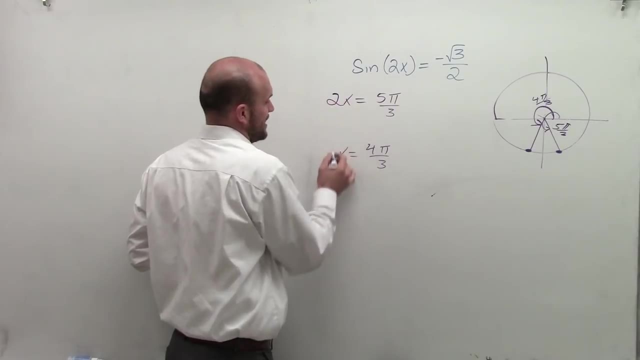 So those are the two angles. when I take the sine of an angle and it's equal to a negative square root of 3 divided by 2.. However, we're not trying to find the angle of just x, It's actually 2x. 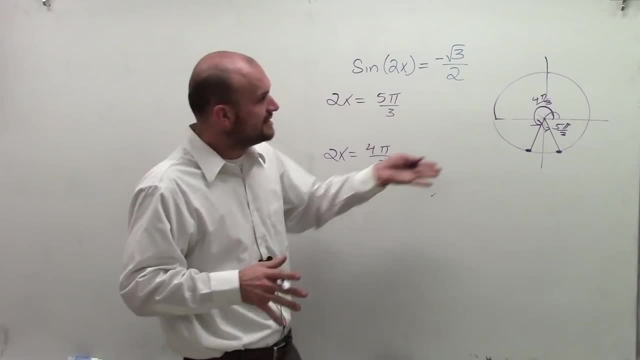 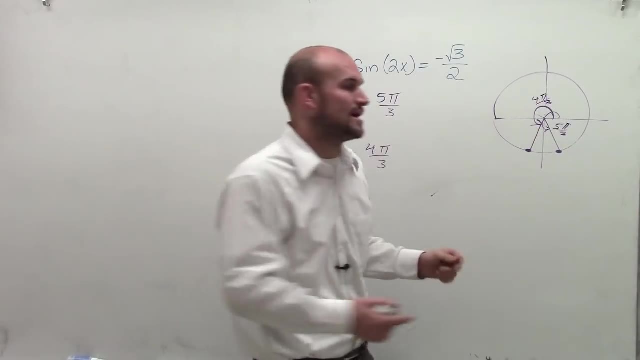 All right, so then, the next thing that we need to look at this is: these are my two angles that are on the interval of 0 and 2 pi. But notice, we want to find all the solutions, So we're going to keep on adding and subtracting our coterminal. 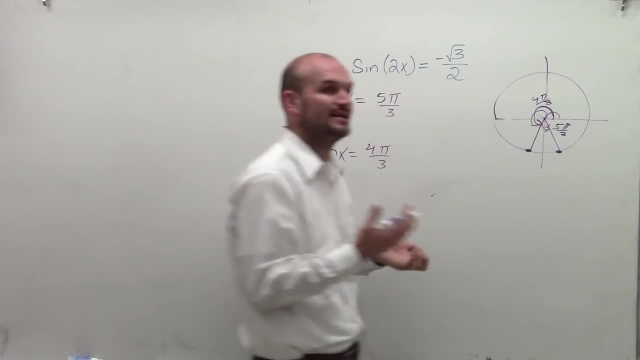 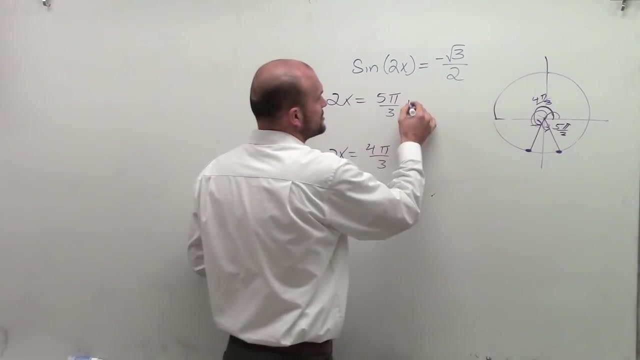 angles, because we can keep on going around and around and keep on getting the solutions of sine being negative- square root of 3 divided by 2, as long as we don't limit it between 0 and 2 pi. So to find my next angle, I can add 2 pi. 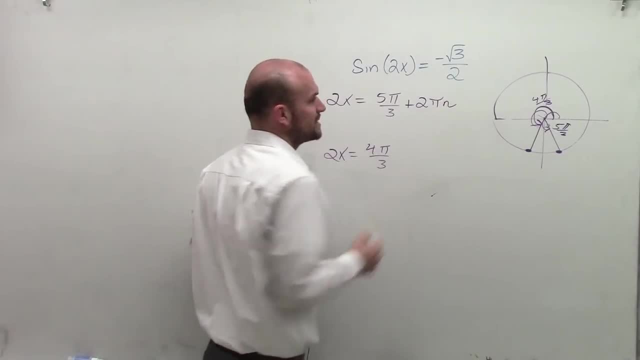 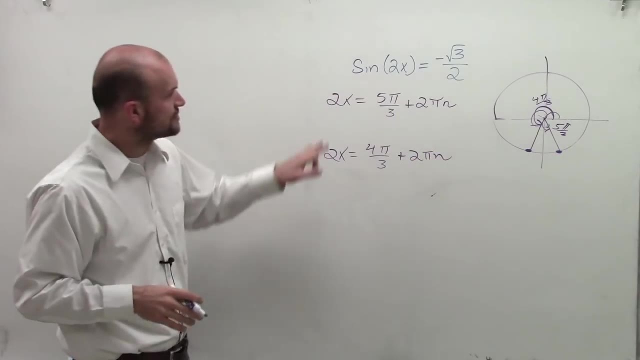 And I can keep on doing this infinite many times, And so therefore I'm going to leave it as a variable. n. Then I can also do the same thing with 2 pi and as well over here. So now to finally solve for x what I'll do. 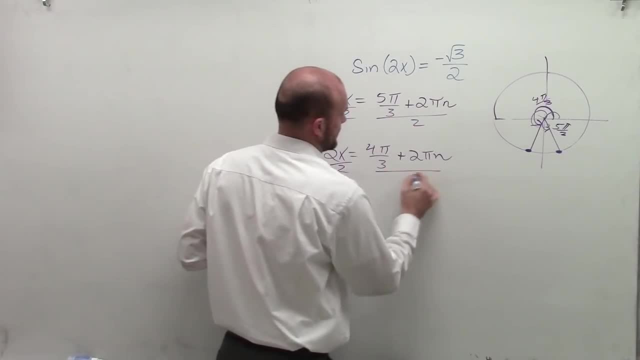 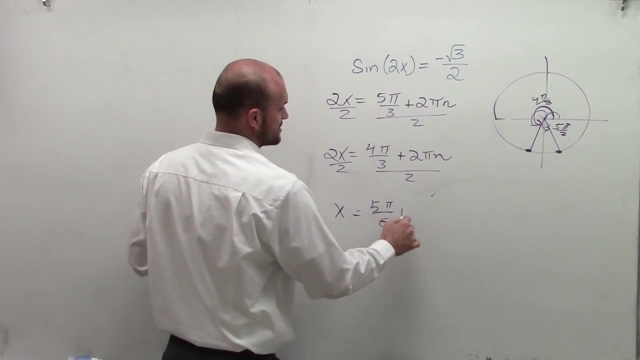 is, I'll divide by 2 on both sides, And therefore my final solutions are going to be: x equals 5 pi Over 6 plus pi n, And x equals 4 pi divided by 6, which we can reduce to 2 pi. 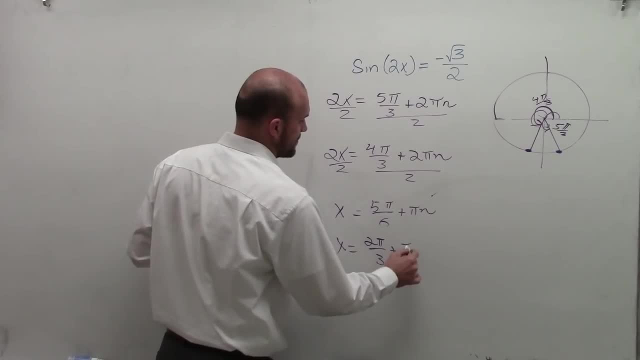 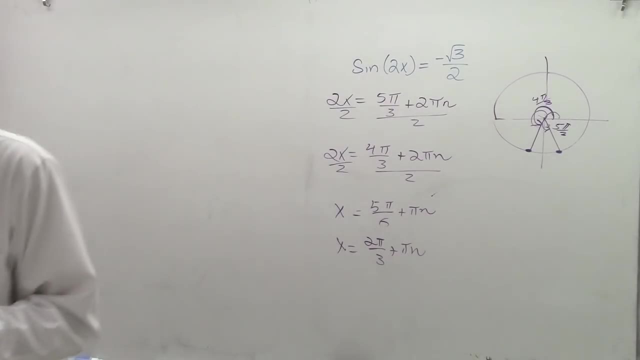 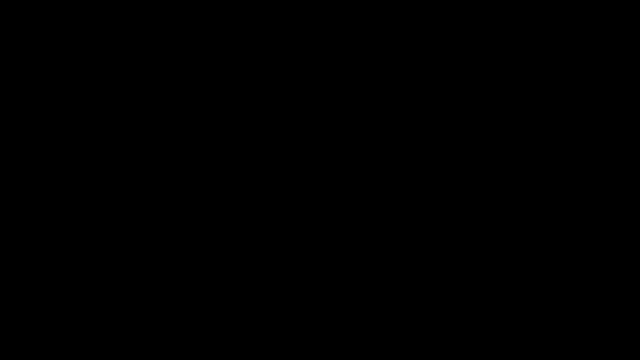 over 3 plus pi? n. So there you go, ladies and gentlemen. That's how you find all the solutions for a multiple angle. Thanks, Thank you. 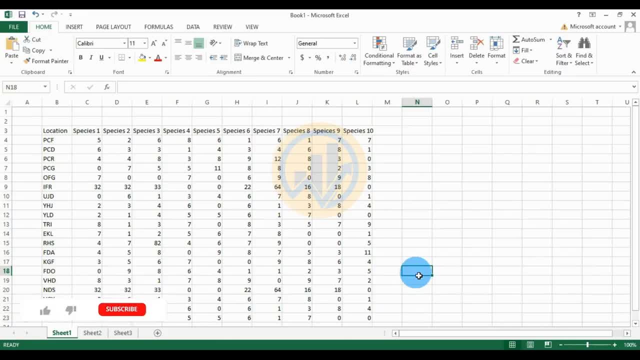 Hi everyone, welcome to statistics bio 7 youtube channel. Today we will discuss topic: how to analyze it for the factor analysis in past statistical software. This is data for the analyzed in the past statistical software for the factor analysis. This is a data set. 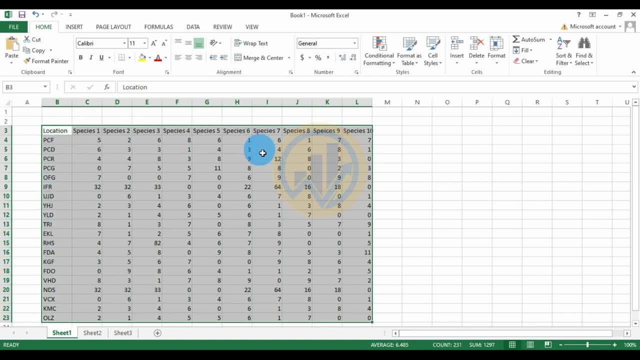 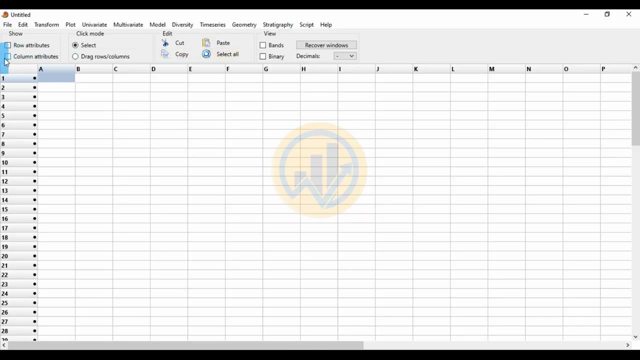 of 15 different locations and the 10 species. This data copied, paste to the past statistical software. First select the data. select the whole the data in the excel sheet, Copy it. Go to the past statistical software and first click the column attributed and the row attributed. 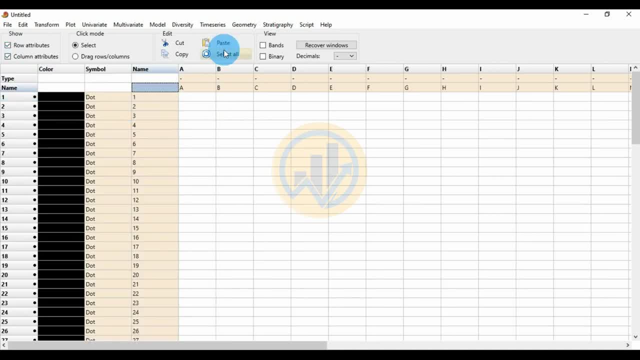 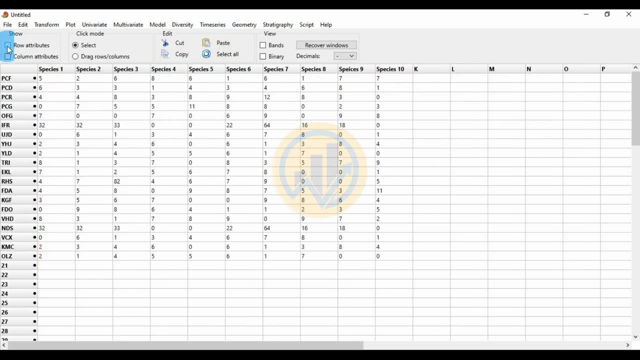 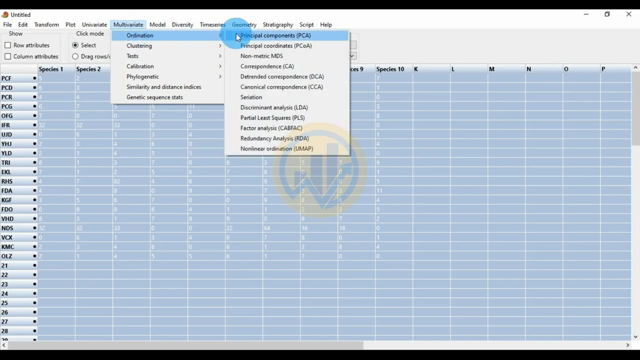 checkbox. Then paste the this column, the data, Click the paste button. Then unclick the column attributed and the row attributed. Then select the whole the data. Go to the multivariated menu and click the ordination button, software, the factor analysis, c, a, b, f, a, c, the factor analysis. then click it. okay, do you want?